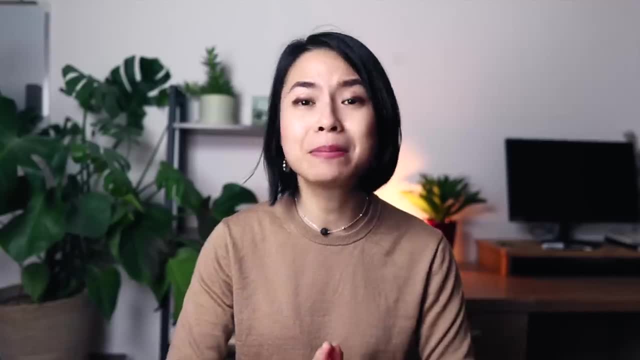 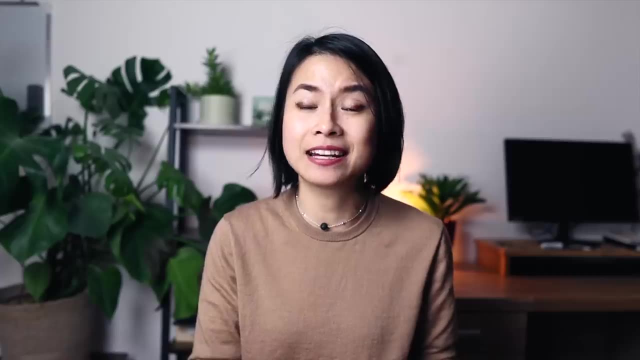 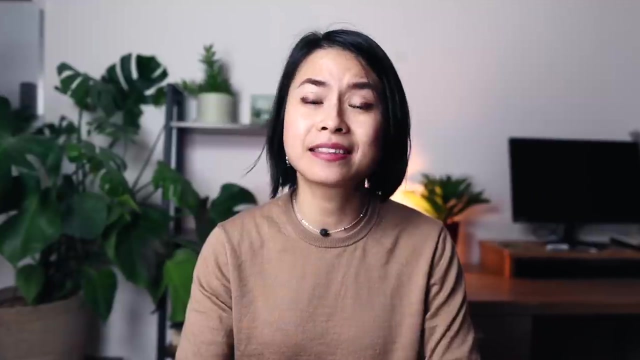 struggle with mathematics and statistics is real for many beginners and experienced practitioners alike. In fact, in some cases you can perhaps get away with not understanding the underlying math thanks to many handy libraries and tools and stack overflow. But understanding math is useful and necessary. 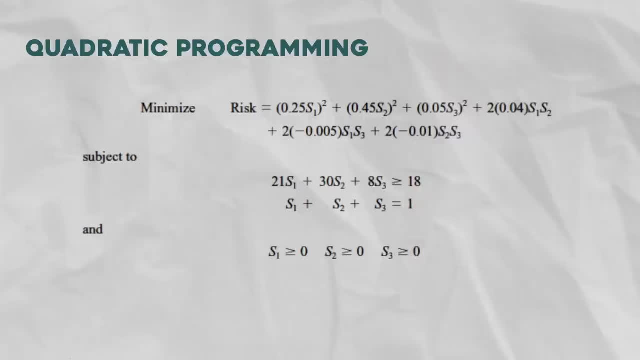 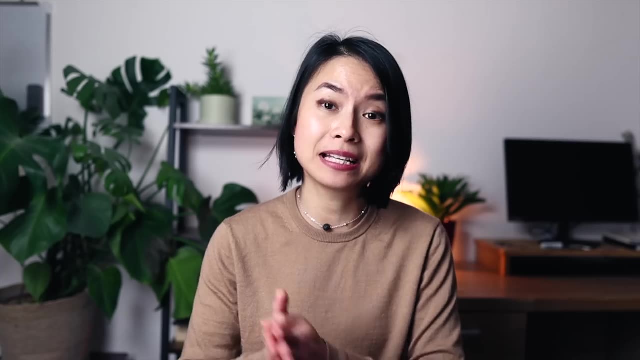 in many cases. A few years ago I had to implement a quadratic programming model in my project, so I had to code up the equation and the input matrices myself. It was all fun and great until I ran into an error that reads like this: 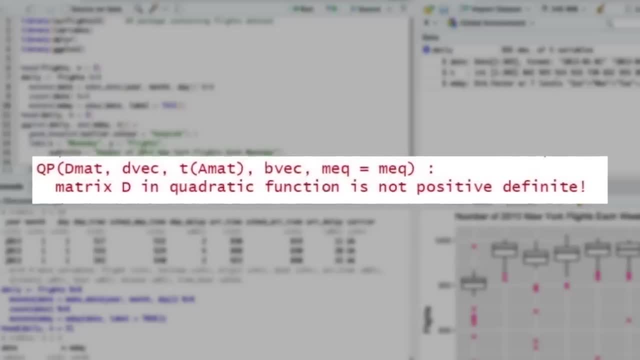 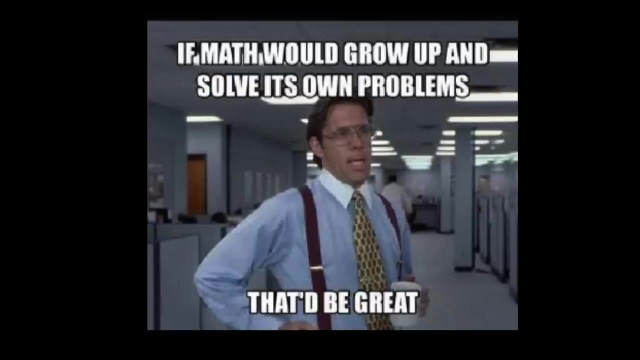 Matrix D in quadratic function is not a quadratic function, It's a positive definite. My linear algebra was very rusty so I had to spend literally a whole day trying to understand this issue and fix it. I think the same goes when you do machine learning. When a 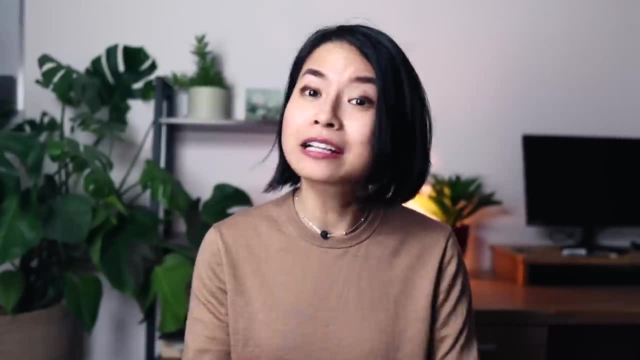 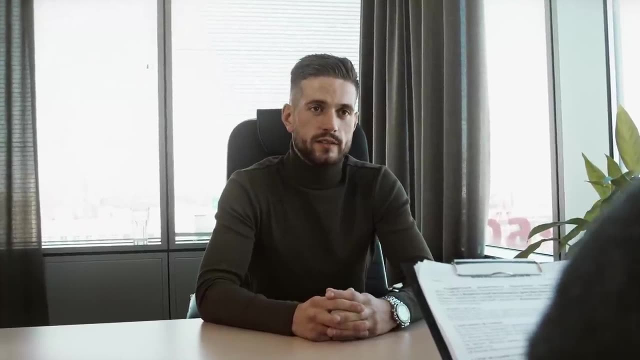 model doesn't converge or something unexpected happens, you actually need to have some math skills to diagnose the issue as well. If you have data science job interviews, solid math skills also give you a lot of self-confidence and generally puts you in a better position. And last but not, 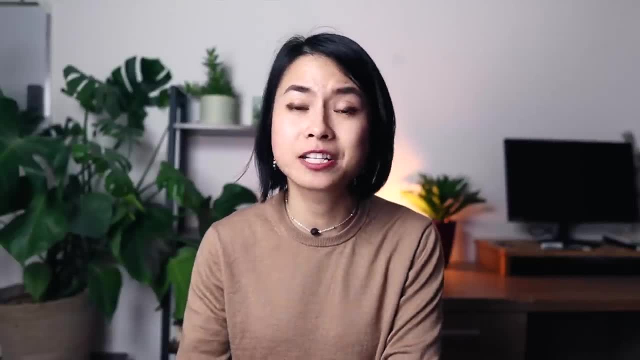 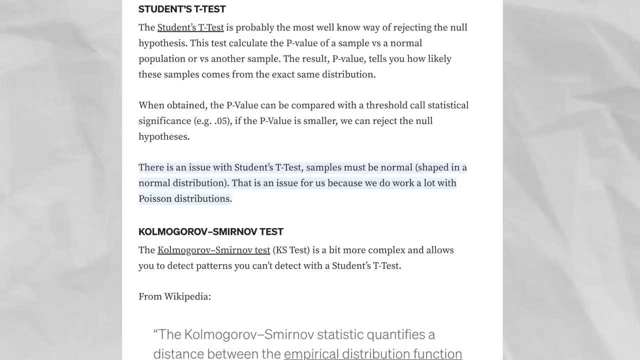 least you'll have the ability to do a lot of work on your own. So if you have a lot of work on your own, you'll have the ability to spot incorrect information or arguments. The other day I came across a Medium article that explains some statistical tests. At one point the article 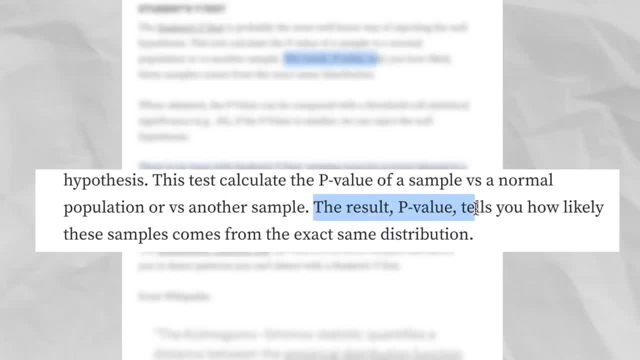 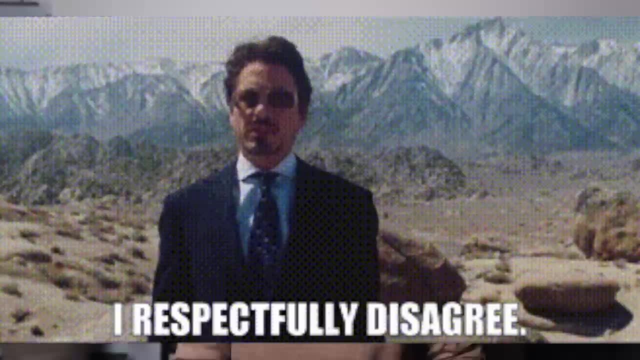 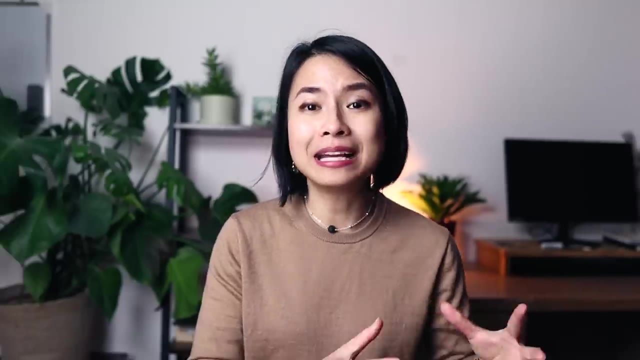 talks about the student's t-test and says something like: the p-value tells you how likely the samples come from the exact same distribution, And this is not correct. The p-value does not tell you if the two samples come from the exact same distribution. It is supposed to tell you if the means of the 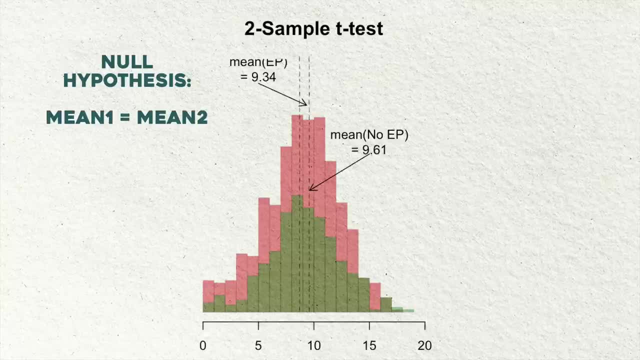 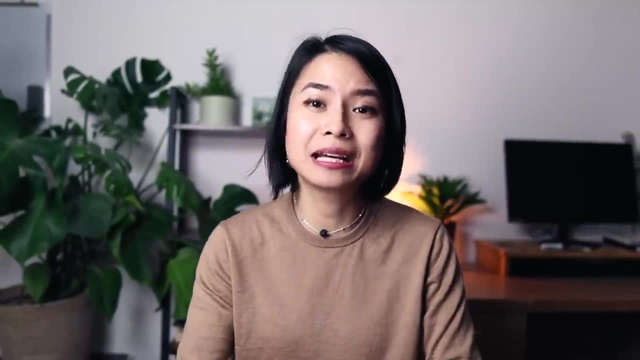 distributions are similar. This subtle mistake is not a good thing. It's not a good thing. It's not a good thing. It's not a good thing. Our understanding can fool anyone, even if they are experienced data nerds. I hope to convince you that we need to have a good foundation in math. 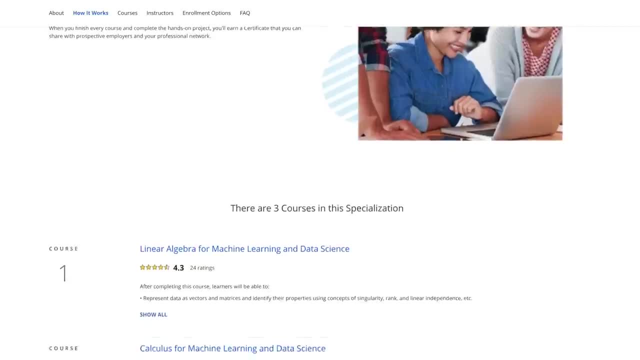 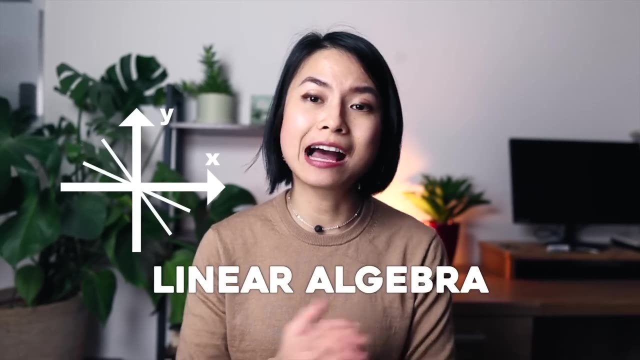 and statistics. So what do we learn in this specialization? There are three courses in this specialization: linear algebra, calculus, probabilities and statistics. The first course, linear algebra, will teach you everything about linear equations, vectors and matrices. You'll 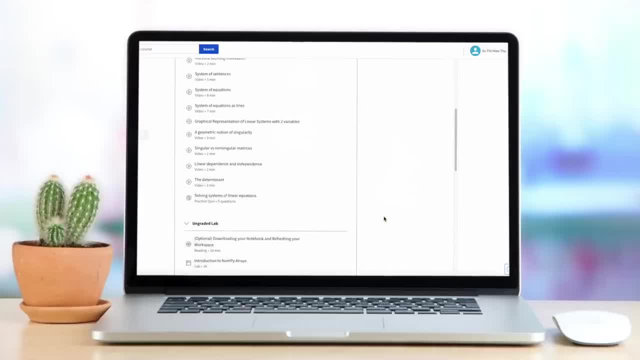 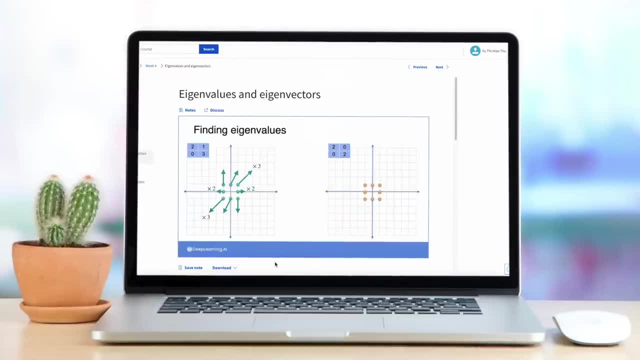 learn concepts such as singularity, rank and linear dependence. Also, you'll learn various operations on vectors and matrices and how concepts of eigenvalues and eigenvectors are applied to machine learning problems. Understanding linear algebra can help you understand better a. 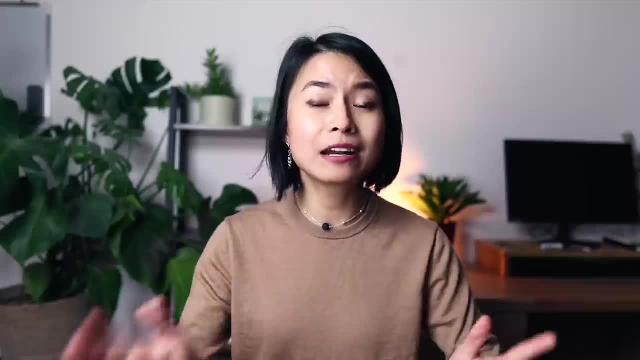 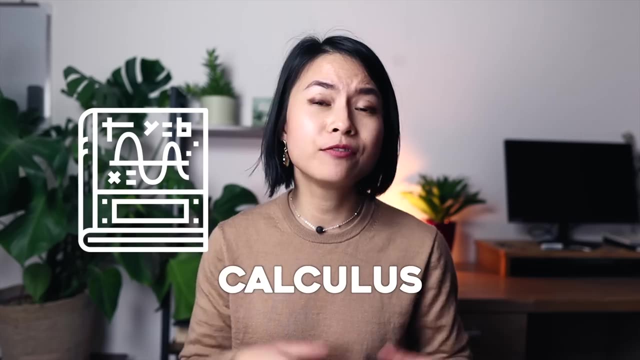 lot of things, from linear regression to neural network. It can also help you make your own algorithms to run more efficiently or converge better. The second course is calculus. If you're one of the people who never really understood why you need to learn calculus in school, this course. 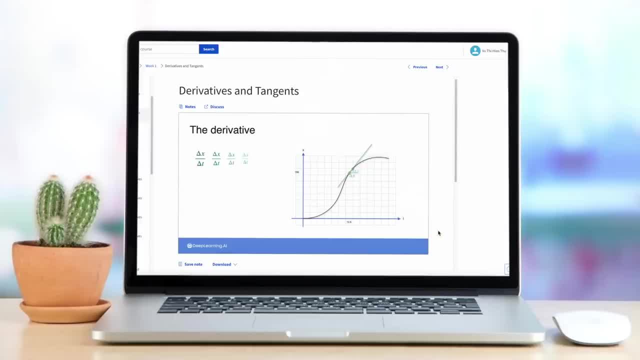 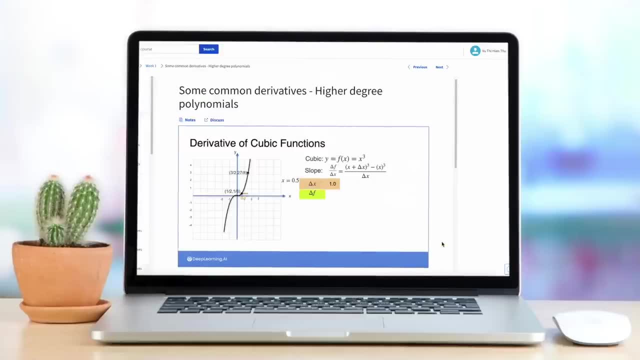 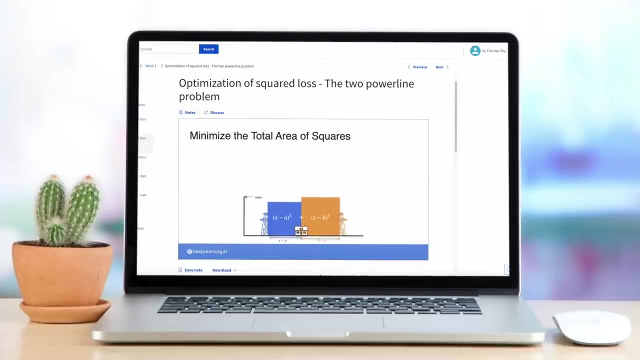 is definitely for you. This course will cover specifically gradient descent optimization algorithm, together with concepts such as derivatives and their properties. You'll learn how gradient descent works in perception models and neural network models. The lessons and the programming assignments will go in depth into how exactly parameters are calculated and optimized in these. 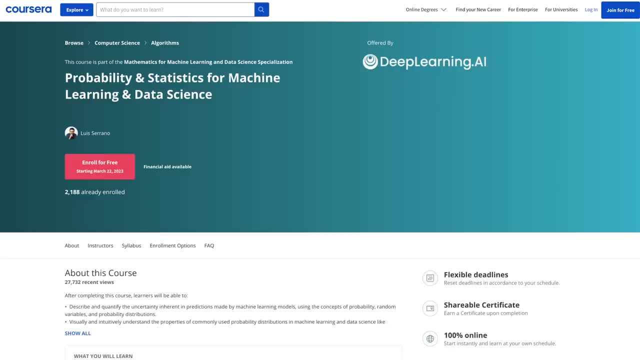 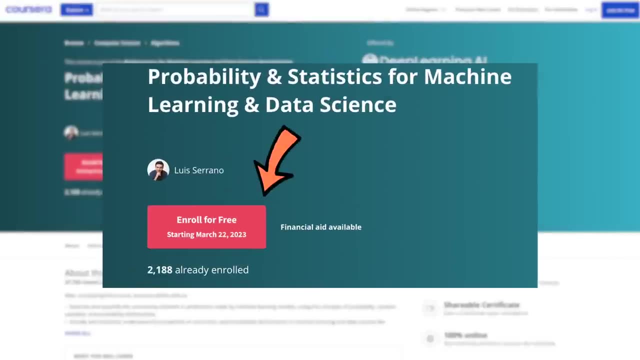 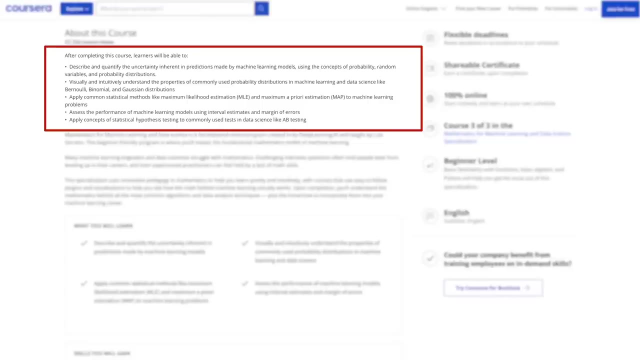 models. The third course is probability and statistics. This is another topic that is broad and scary For a lot of people. this course is unfortunately only started in March, so I can't give you an insider look into the lessons, but this course covers all foundational topics such as probability. 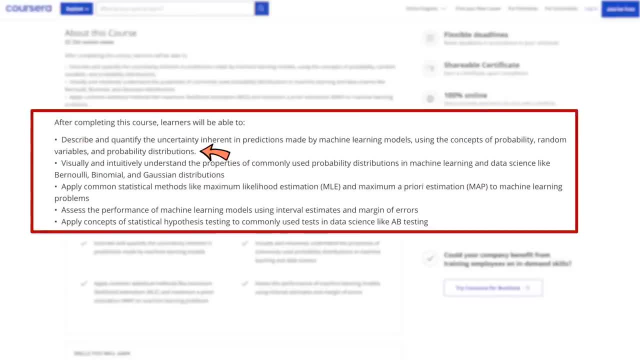 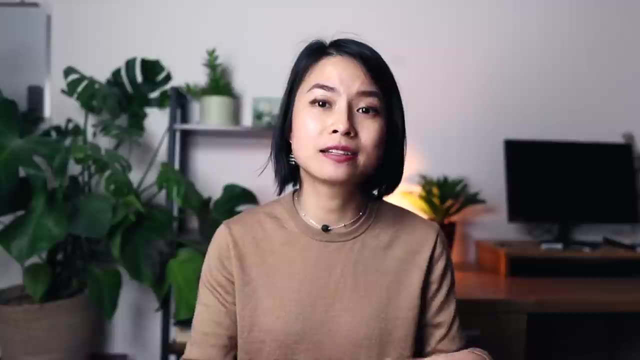 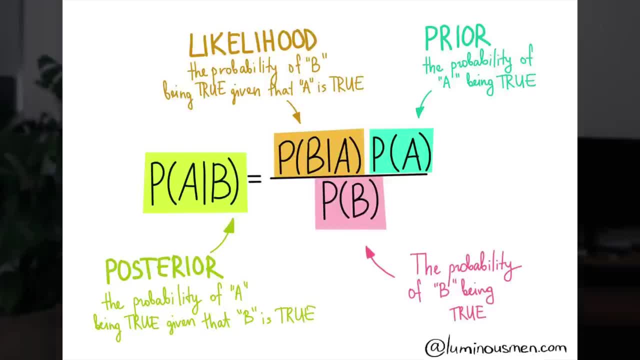 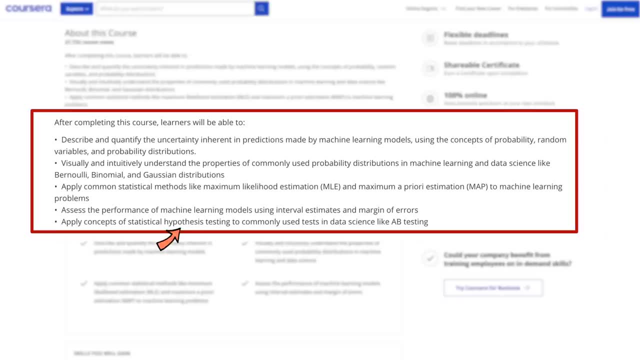 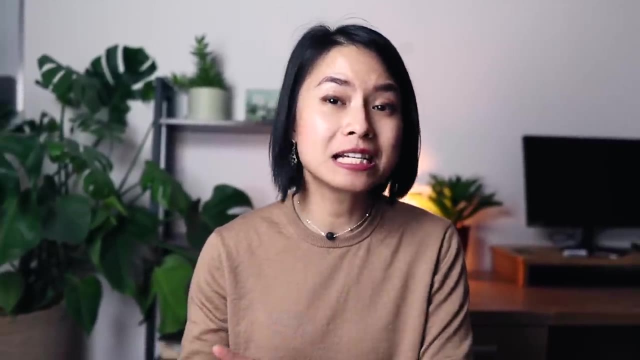 likelihood estimation or using Bayesian estimators. These concepts will also be explained in this course. Finally, you'll learn about hypothesis testing and assessing model performance using statistical methods. These are all very essential topics in data science in general and machine learning in particular. In my job, I sometimes do model validation for statistical 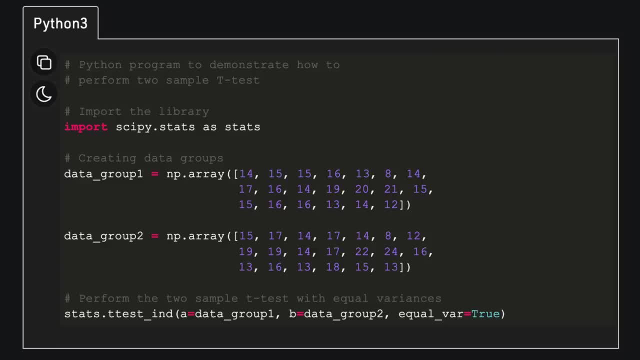 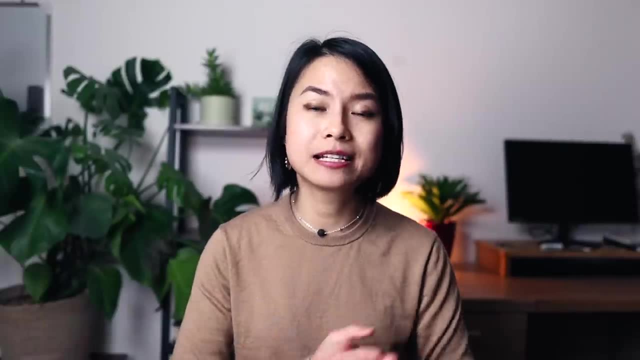 models. so understanding statistics and how to perform t-tests, for example, is a must-have skill if you want to be a good model tester, If you want to be a good model tester. you need to be a good model tester if you want to assess and challenge a model On Coursera page. this specialization 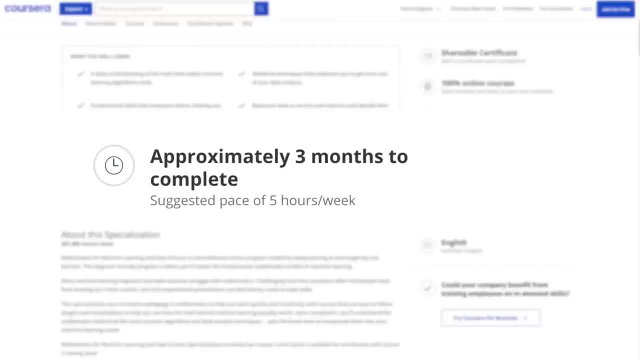 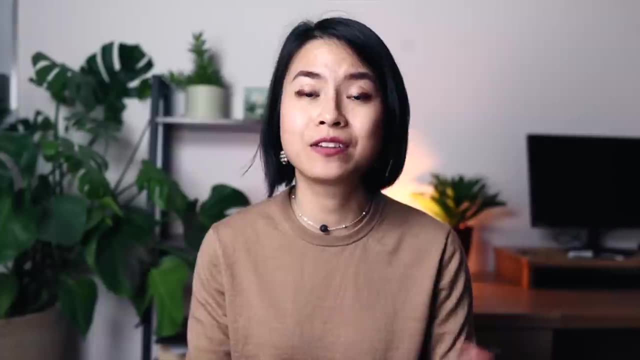 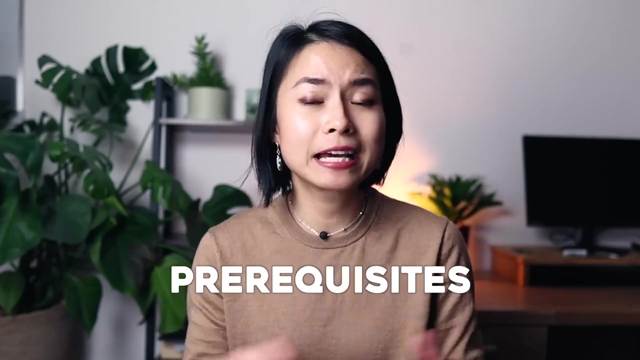 takes approximately three months to complete if you study five hours a week. So even if you are working or studying full-time, I think it's totally possible to fit it in your evenings or weekend schedule. This is supposed to be a beginner-friendly course, so in terms of prerequisites there's not. 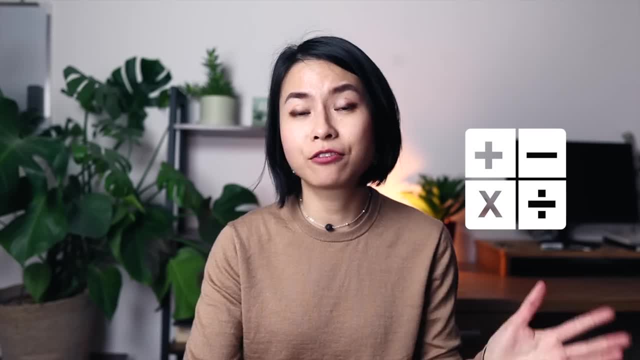 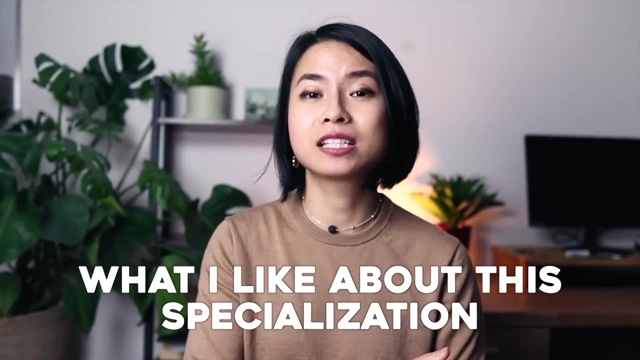 much to worry about. It is just recommended that high school level mathematics will be enough to help learners get the most out of their studies. If you're interested in learning more about this specialization, I'm sure you'll find it helpful. Now, moving on to what I like about this. 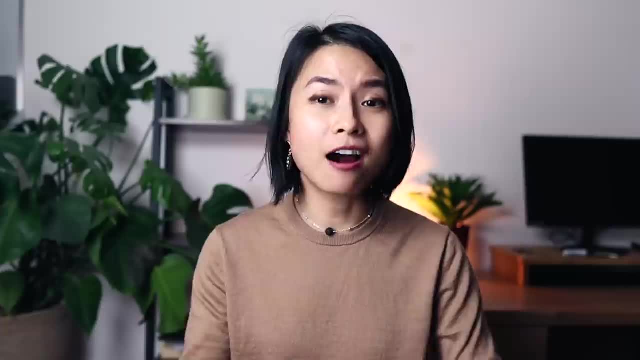 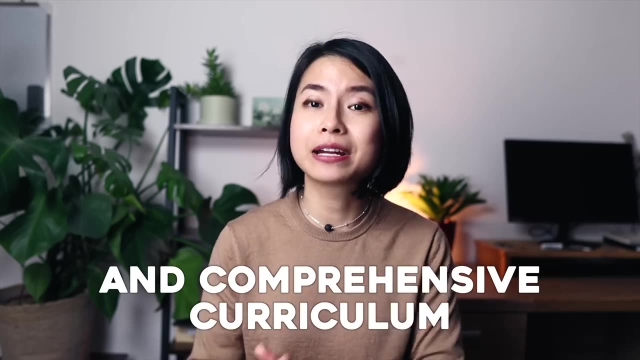 specialization and what I might not like as much. There are many things to like about this program. Firstly, I think it has a very well-structured and comprehensive curriculum. The program stays close to the most useful concepts for data science and machine learning. 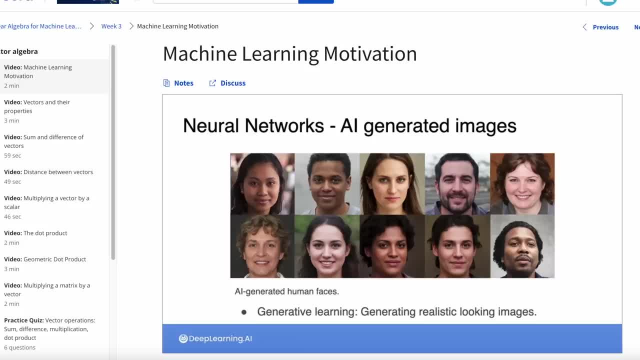 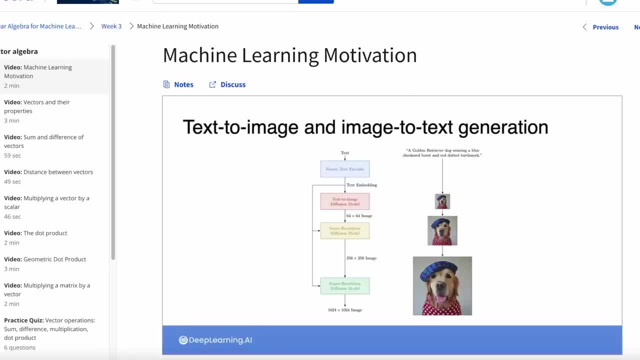 which is not the case in other general math courses. Each week's lesson starts with a machine learning motivation example, which explains why and how the concepts at hand are a must-have for students who are interested in learning more about data science and machine learning. 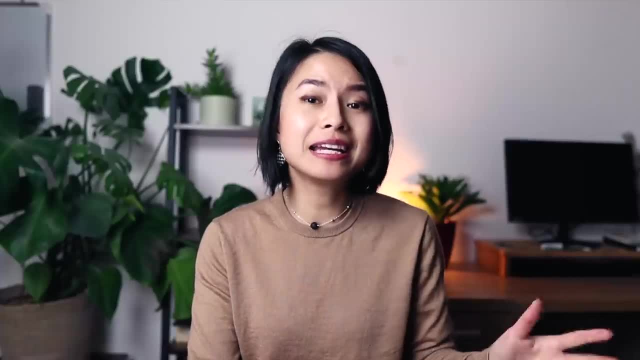 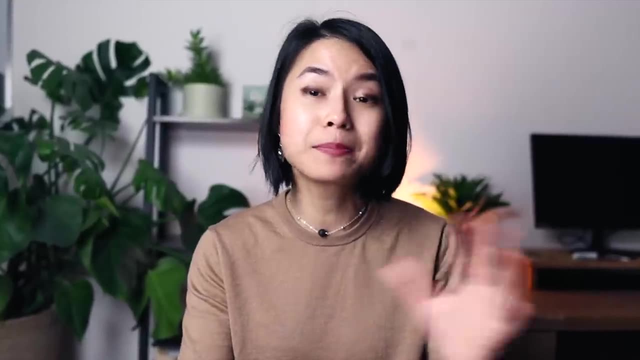 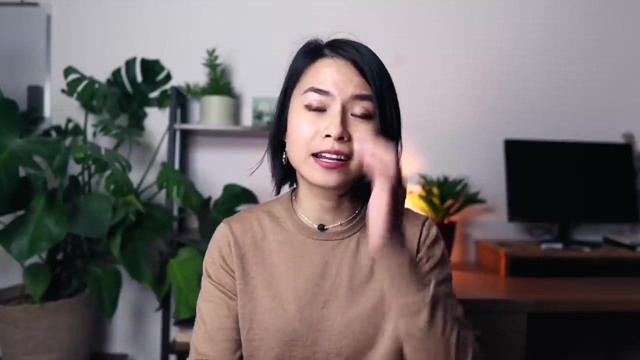 Also, the topics are discussed really in-depth and from ground up, so you don't need to worry, if you like, any pre-existing background or experience beyond basic high school math. so I believe it will help you build a very good conceptual understanding that sharpens your intuition. 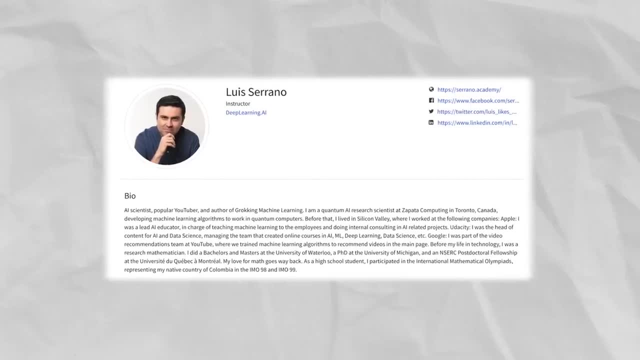 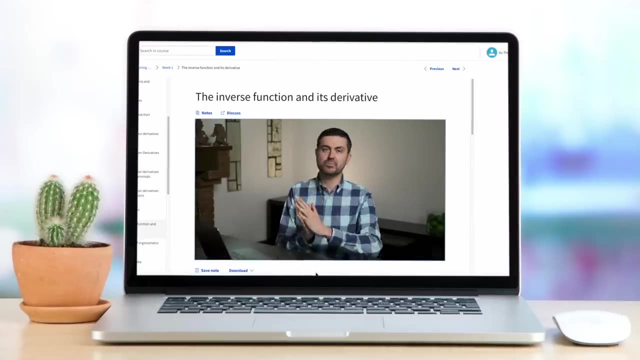 when doing data science. The program is taught by Luis Serrano. I hope I say his name correctly, so not Andrew Ng. At first I was a bit upset about this, but Luis Serrano also has a very engaging teaching style and his delivery is very concise and easy to follow. 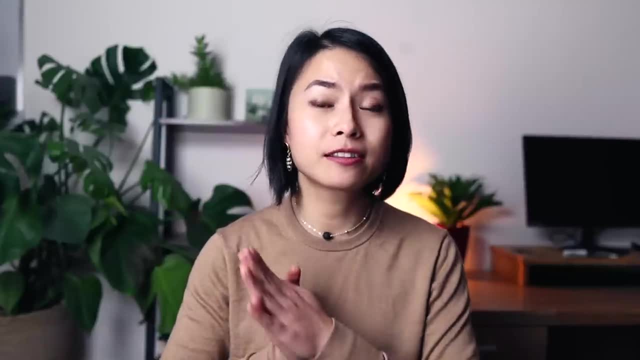 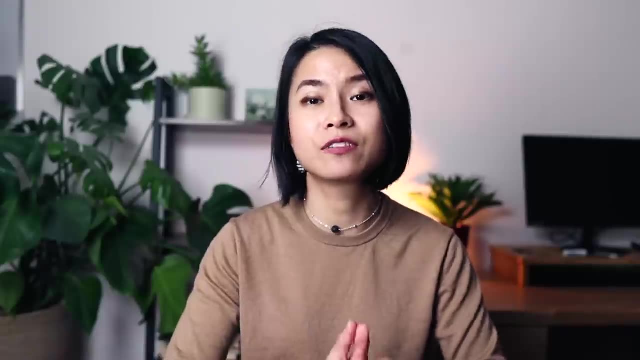 So, yeah, you really can't complain much. In addition, the lectures have interactive visualizations and you can really tell how much effort has been put into making those visualizations. I really think the team has done a great job in making the explanations. 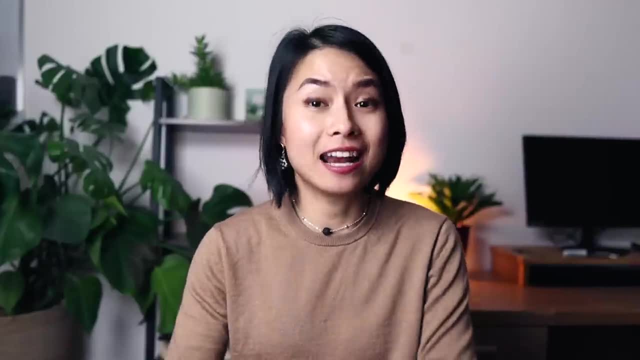 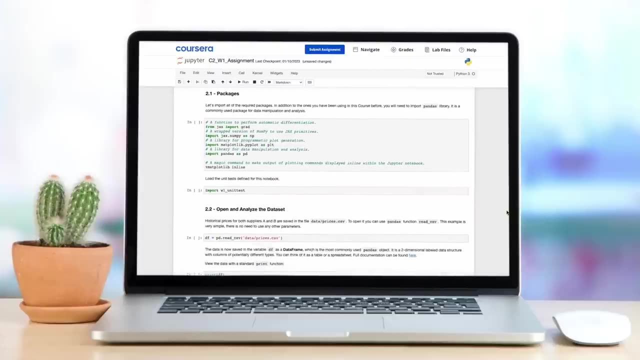 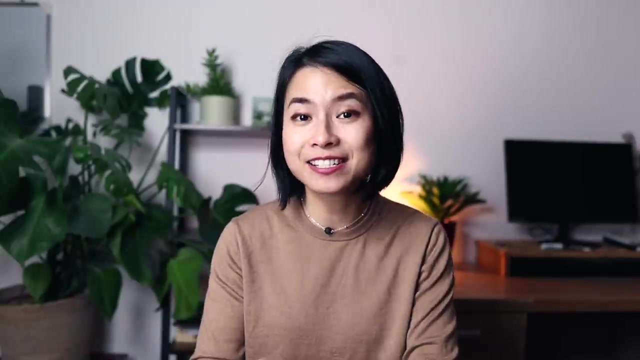 more intuitive with those visualizations. Another thing I like about this program is the hands-on programming assignments. Each week you have a programming assignment to work on. They are all in Python and you can work on the lab environment on Coursera, so you don't even need to have Python installed to be able to work on the assignments. 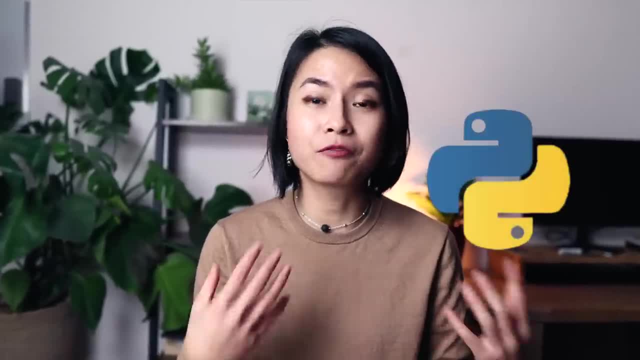 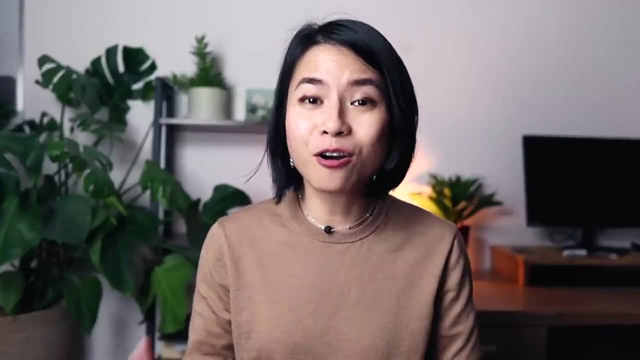 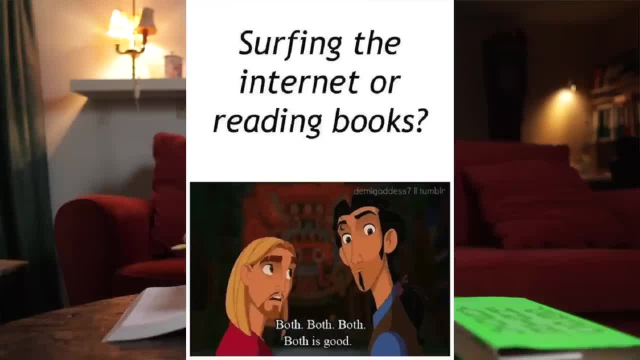 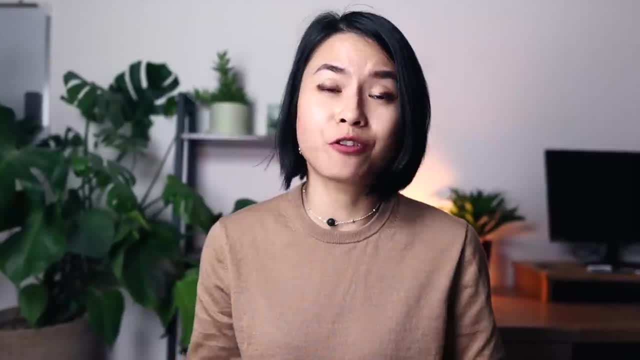 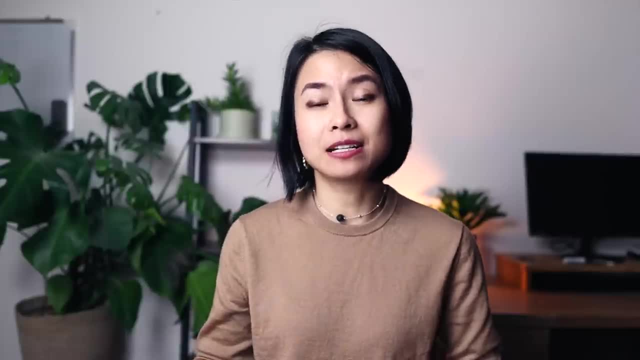 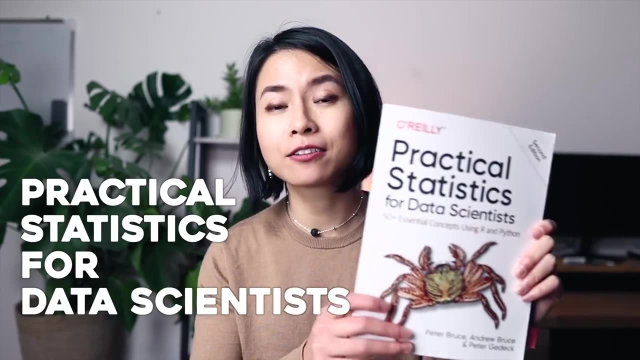 Because of this, I'd highly recommend you combine this specialization with some books to make the most out of the course. One of the books I found really helpful for beginners is Practical Statistics for Data Scientists. This book covers the same topic as the third course of the program. 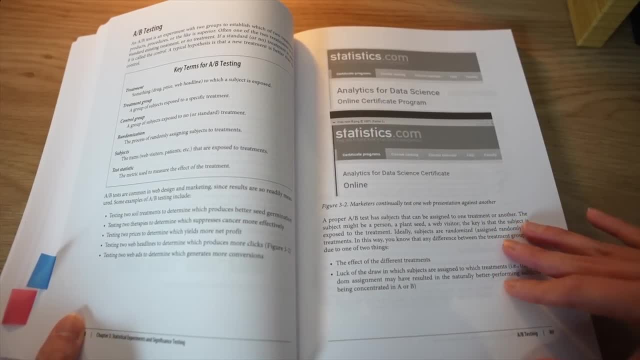 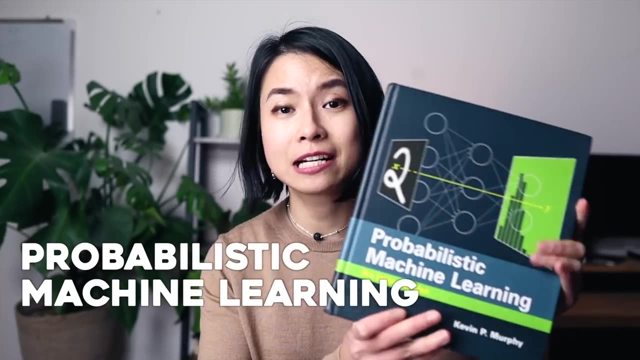 on probability and statistics so you can refer to this book for further reading. A more advanced book you can use for this whole specialization is Probabilistic Machine Learning. This is really the best book that I've come across for theoretical understanding of machine learning. 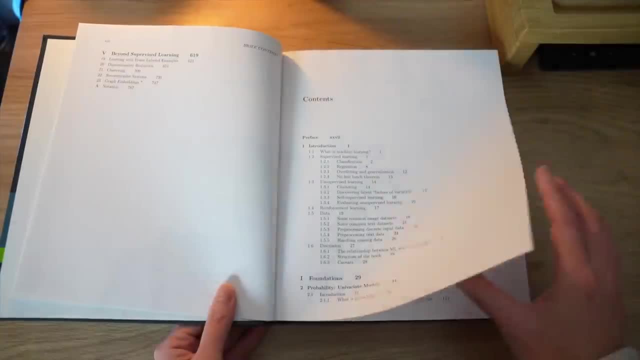 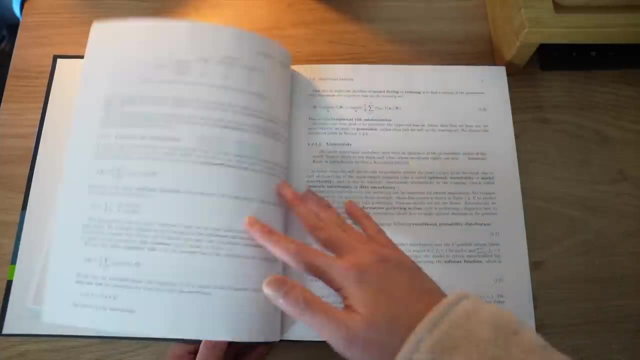 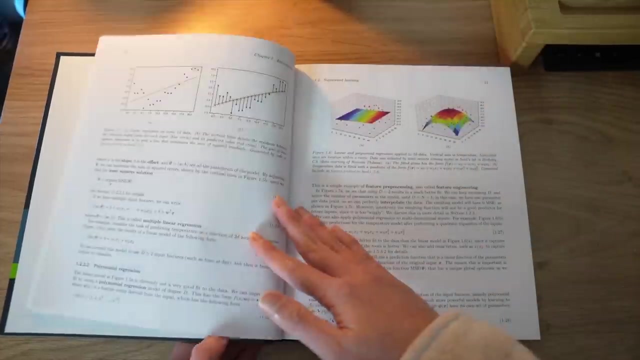 algorithms. The first chapter of this big book is fully dedicated to the basics of linear algebra, probability, statistics and optimization. It also familiarizes you with the common math notation, which is really helpful. if you want to read machine learning research papers, You will find 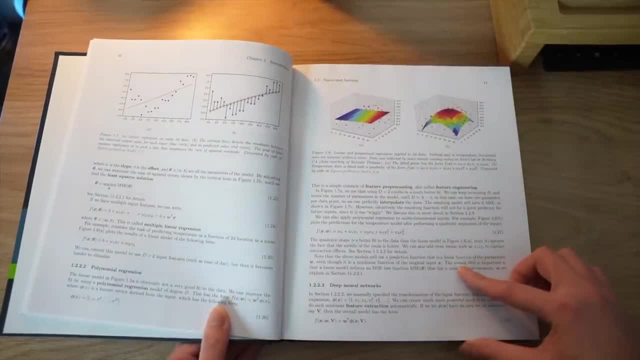 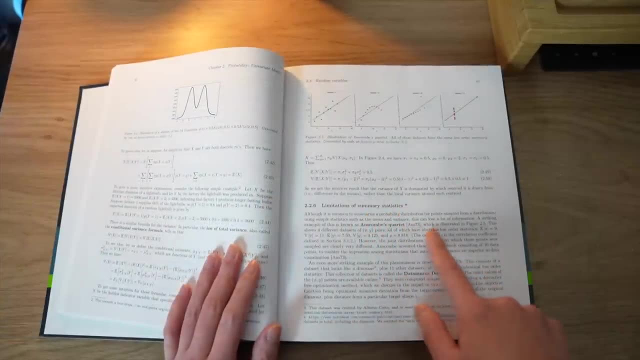 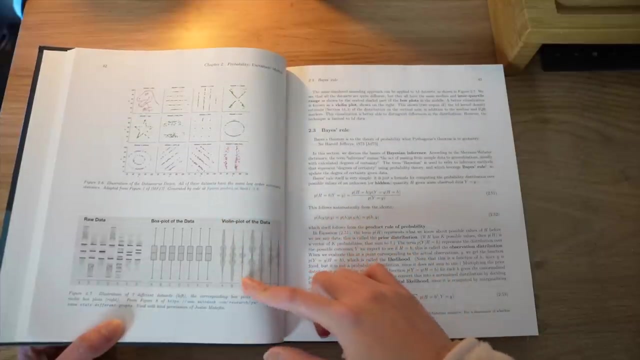 here a lot of nuances to these topics which might not be covered in such extent in this specialization. For example, here it's talking about why we might still lose a lot of information by describing distributions with basic statistics like mean and variance. There are a lot of pictures. 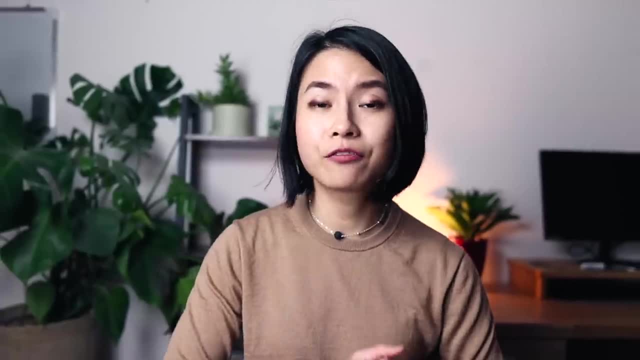 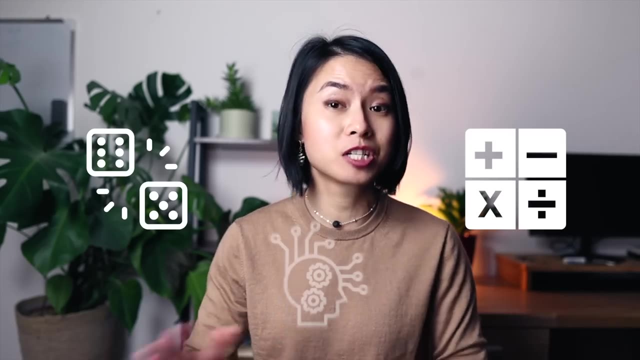 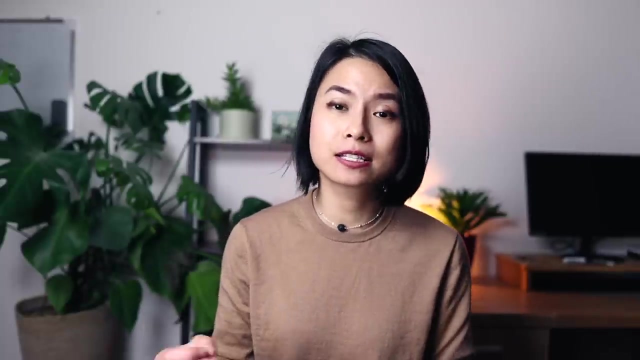 and examples in this book, so I think it's a great reference material for someone who wants to develop more in-depth understanding of math, statistics and machine learning algorithms. So let's talk about whether I'd recommend this course and to whom I think I'd highly recommend this.